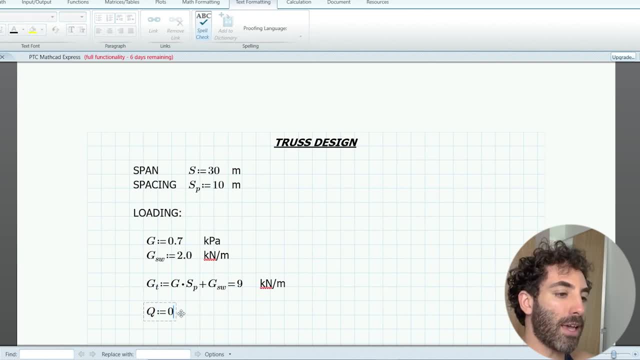 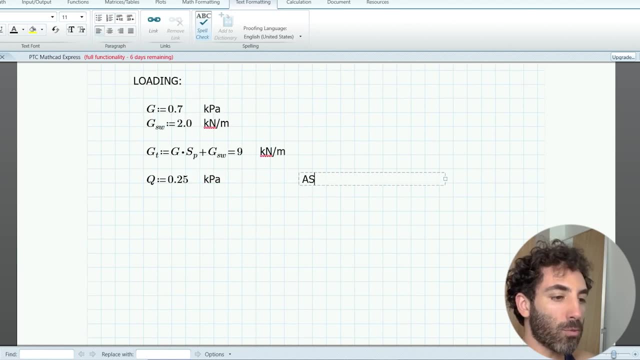 per meter and the live load is 0.25 kpa and that comes from as 11, 70.1, page 13, table 3.2. and now we need to transform kpa to kilonewtons per meters, and therefore 0.25 times the spacing. 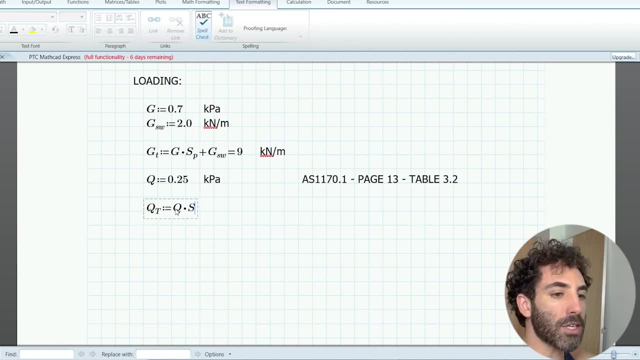 and that gives us 2.5 kilonewtons per meter. okay, so far nothing difficult. we had to find the loads in kpa and transform to linear distributed loads. so the next step is the load combination. so to design for strength, which is usually the load combination. 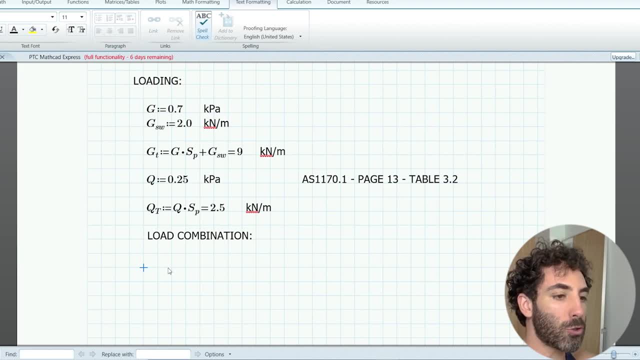 usually bending shear, compression and tension. we use ultimate limit state and w? u l s. so that's the ultimate uls is the ultimate limit state and we're going to use w? u l s. that will be 1.2 times g plus 1.5 times q and that's the load combination which is equal to: let's see: 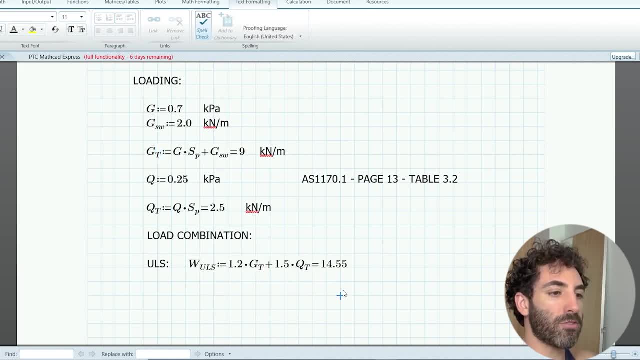 here. let's just fix it. this number, 14.55 kilonewtons per meter. now for the serviceability design we use. the service limit states, which is the w s, l, s equals to g plus 0.7 q, and that equals to 10.75. 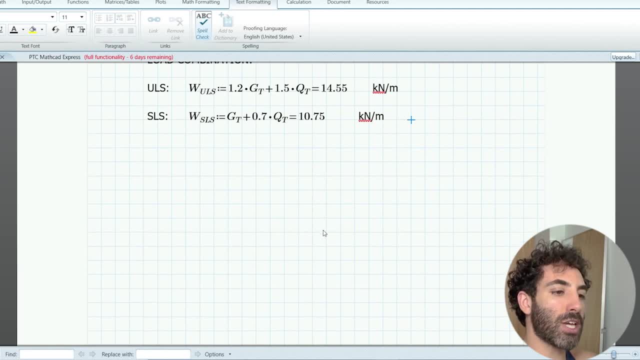 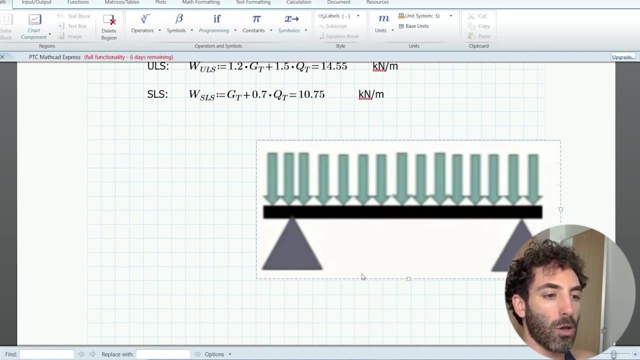 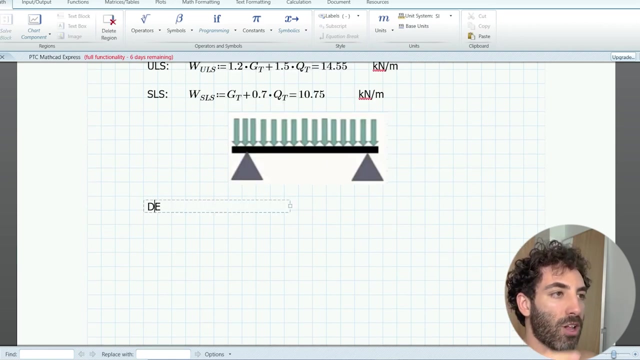 kilonewtons per meters and we use this combination to check deflection and vibration. for our case, we won't check vibration because there won't be anyone walking on the roof, hopefully. and speaking on deflection, we need to find the deflection limit, which, in this case, i'm going to adopt: span divided by 300. 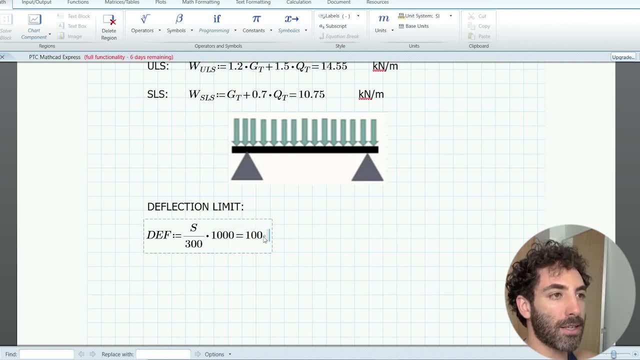 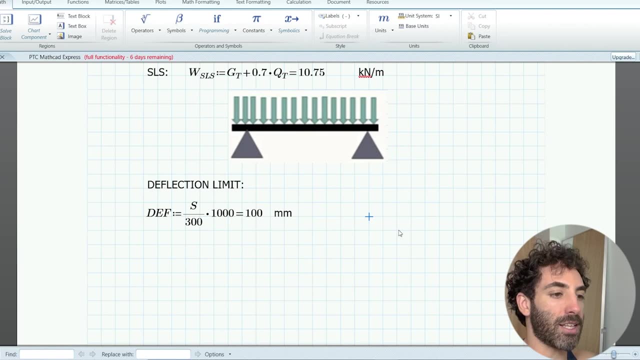 times a thousand. to transform to millimeters, that is equal to a hundred millimeters. you can find a suggested criteria on as1170.0- as1170.0, page 28, table c1, and at the same time make sure to check with the roof sheeting manufacturer. 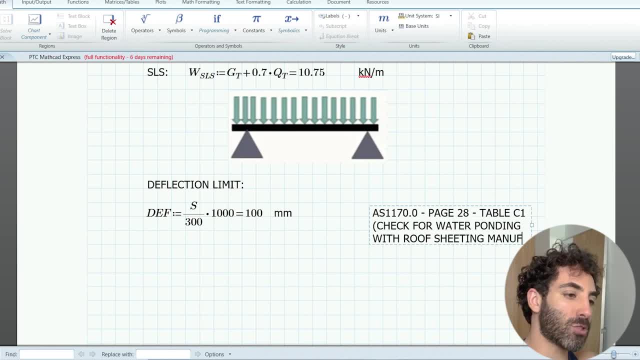 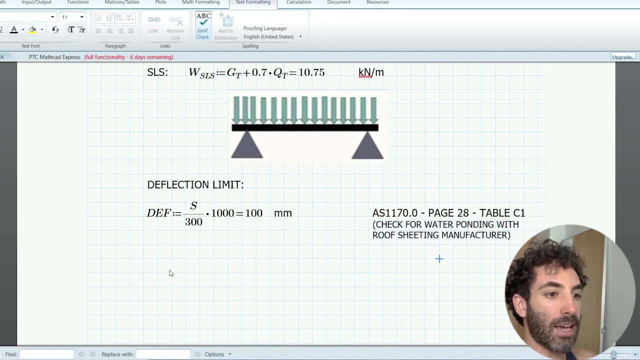 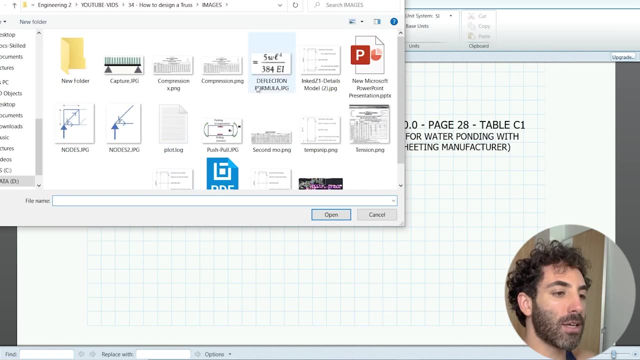 the limits to avoid water ponding, so you might have to set a different deflection limit and you you also don't want people to freak out with massive sagging, so make sure you pay attention to these limits. so the formula for deflection is five times. 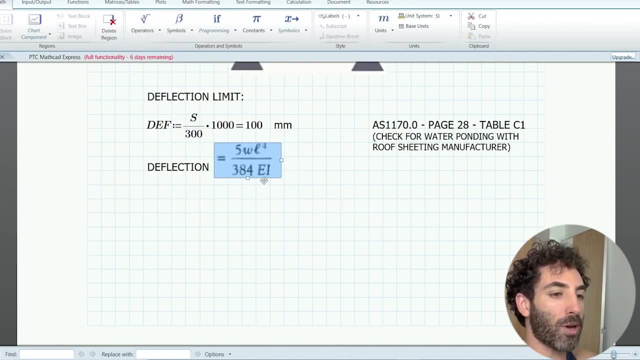 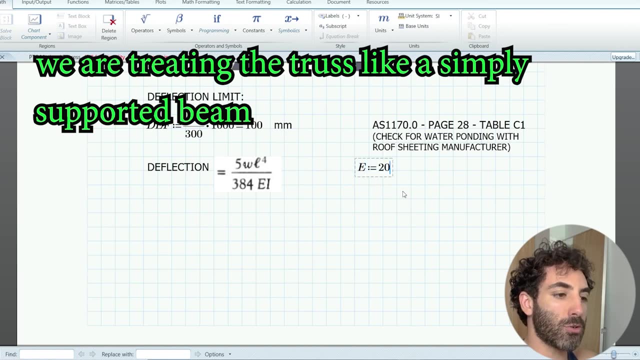 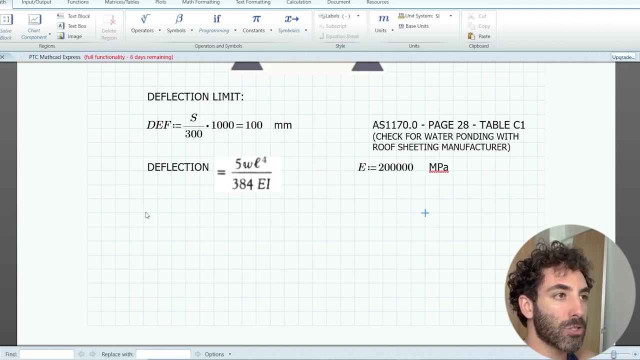 the loading times, the span to the fourth divided by 384 times young's modules of steel, times the second moment of area young's modulus of steel is the measure of the material stiffness, and we're dealing with 200 000 mpa. so now the only unknown variable of this equation is the second moment of. 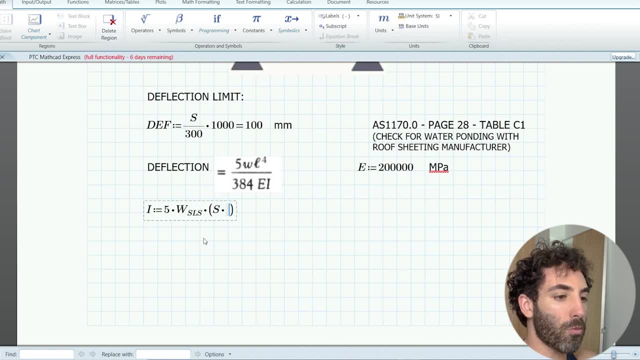 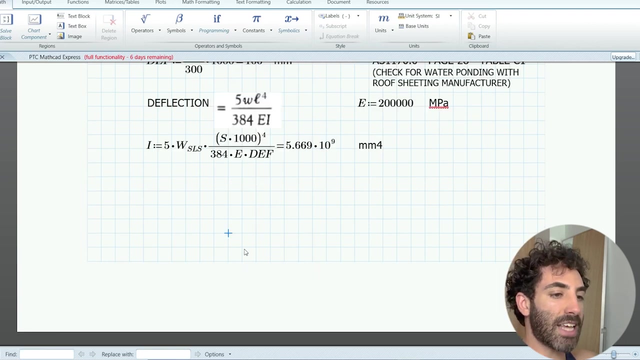 area i. so i'm going to rearrange this formula to work out. i let's do this one here. there you go. i is equal to 5.66 times to 10, to the 9th, millimeters, to the fourth, and the next step is to choose the steel section that our truss will be made of. okay, so? 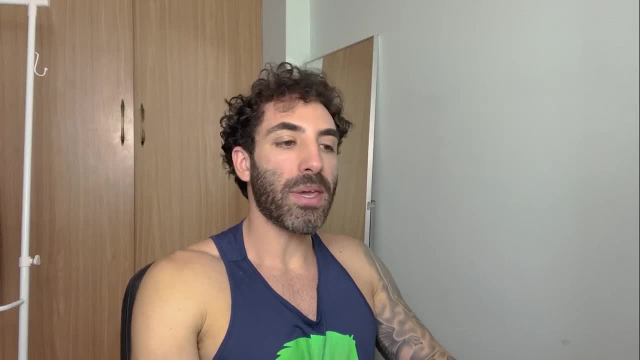 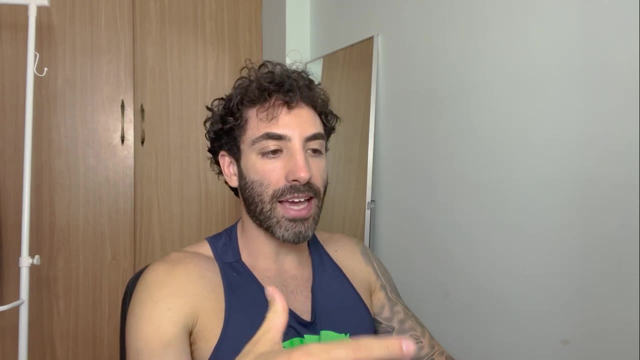 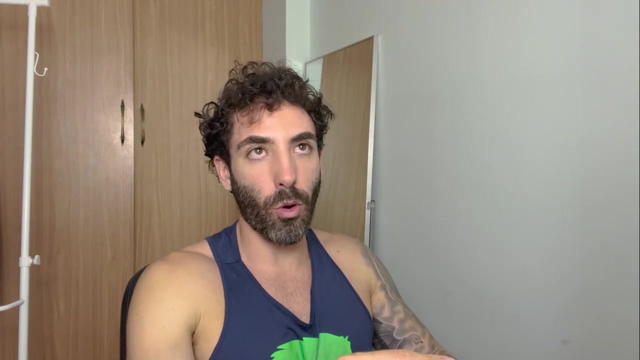 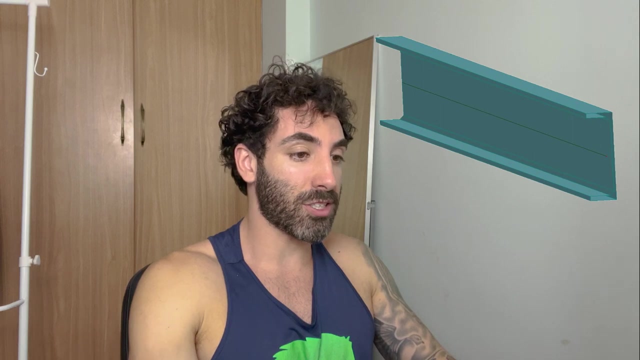 we can make a truss with angles. pfc's uses shs. you should choose a section and think about how hard the connections will be to fabricate and in terms of connections, you can either have a welded or you can have bolted fixings. so for our example, we're going to go with pfc's, which are relatively 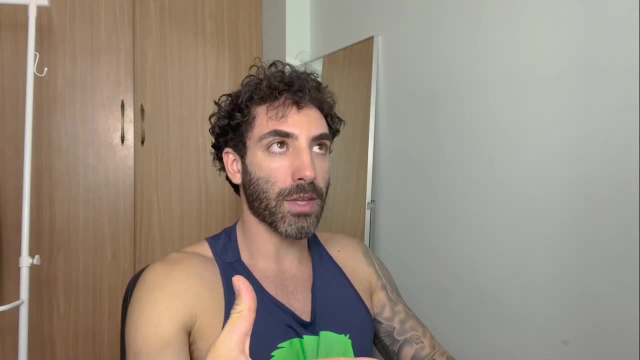 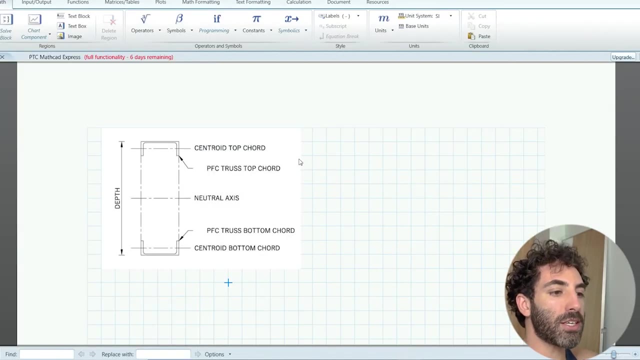 easy to connect and work with. we do a lot of trusses with shs as well, but in this case we're just going to work with the pfc's and what we're seeing here is the cross section of our truss and notice that the pfc's are lying flat. so the 3d would be something. 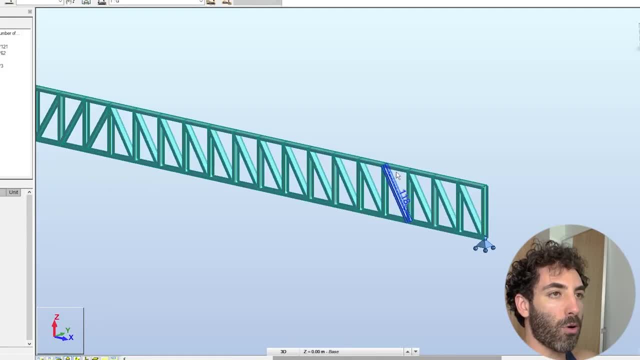 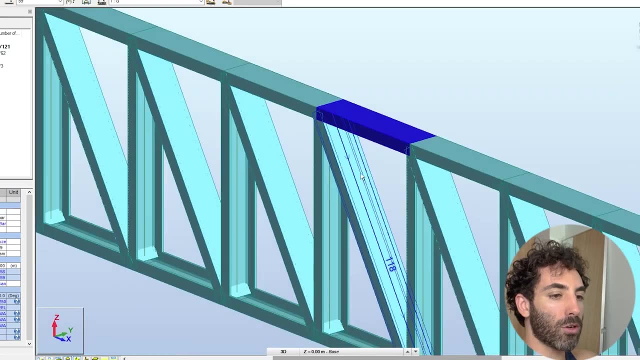 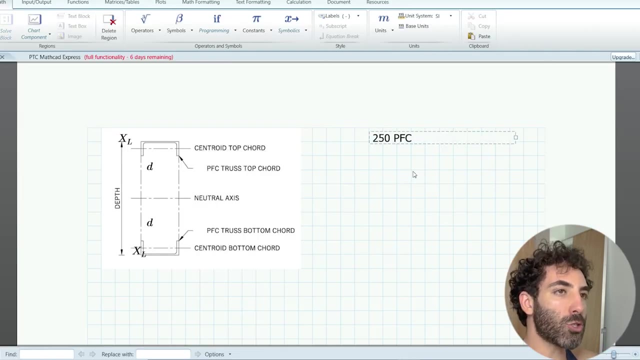 like this, so you can see that the top chord, the top chord pfc, has its flanges pointing downwards and the bottom chord pfc has its flanges pointing upwards. and we will start with a 250 pfc and check if it works. so the second moment of area of a 250 pfc. 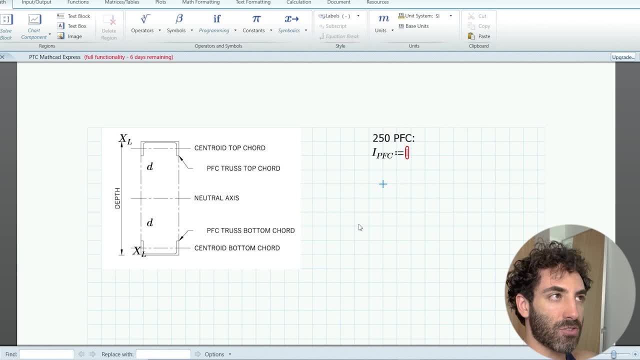 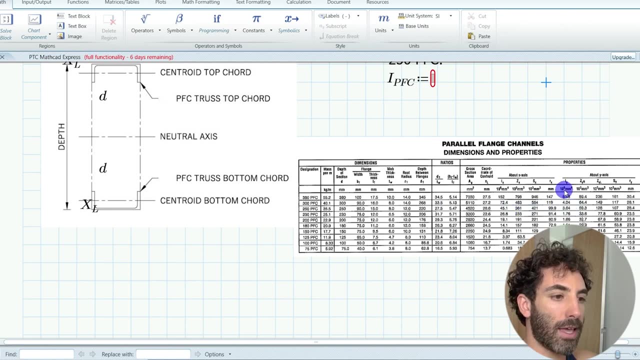 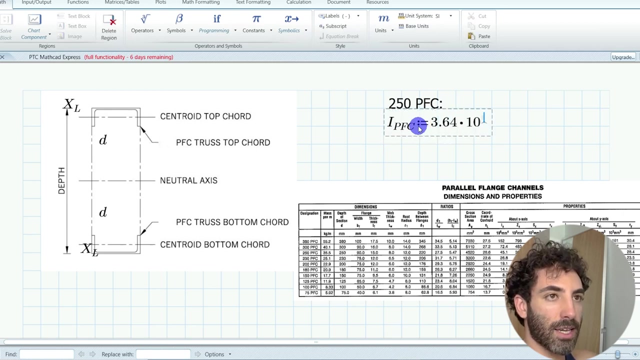 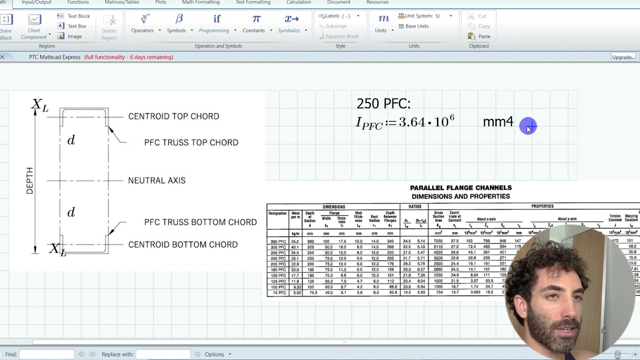 let's find a table that we can get these values from. so the parallel flange channels dimensions and properties, and the i value is 3.64 times 10 to the, and we are, that's millimeters to the four, and we are dealing with i, y. okay, so that's y axis as the 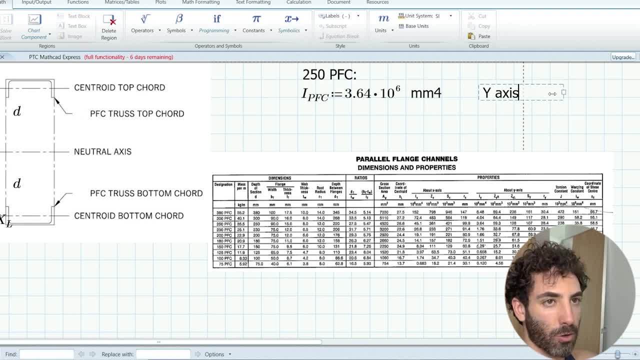 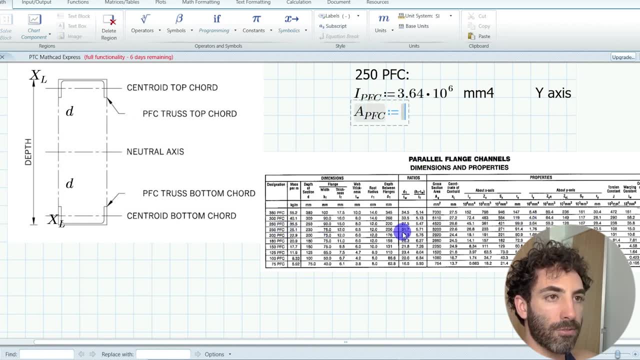 pfc is on its flat- so make sure you don't mix that up- and the area of the pfc is 4520 square millimeters. there we go. let's change that to two, and the centroid distance x- l is 28.6 millimeters. okay, since this is a built-up section, we have to use the parallel. 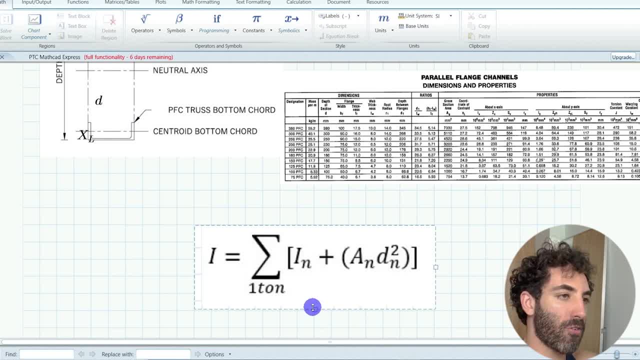 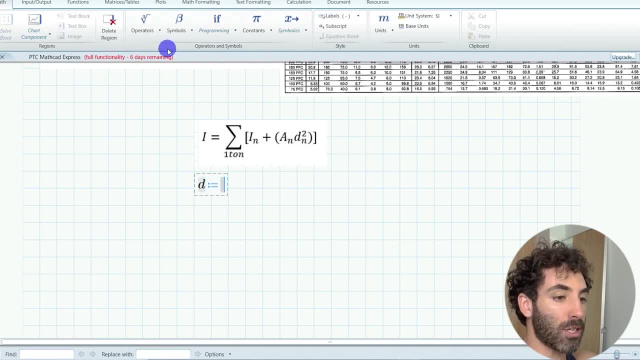 axis theorem, and you must have learned this in your physics classes. so we're going to rearrange this equation to find the little d, which is the distance from the centroid of the pfc to the neutral axis of the truss. remember that this section is symmetrical. therefore we're multiplying everything by 2. 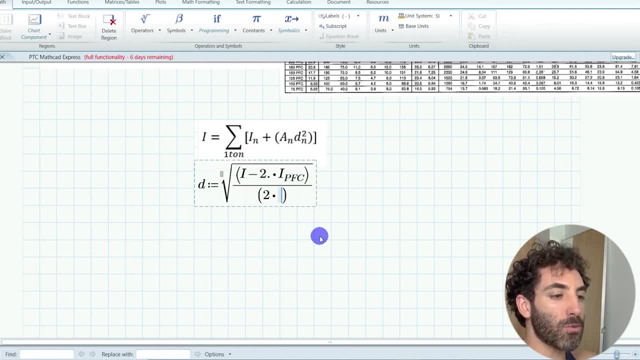 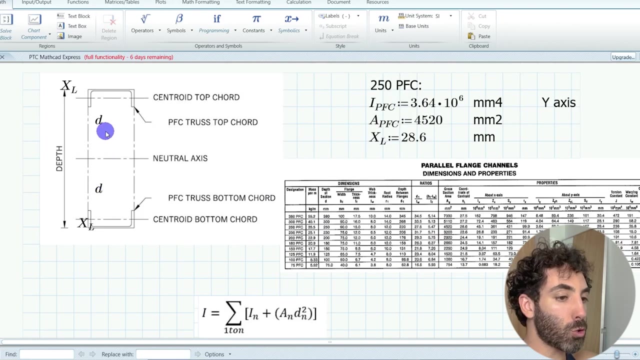 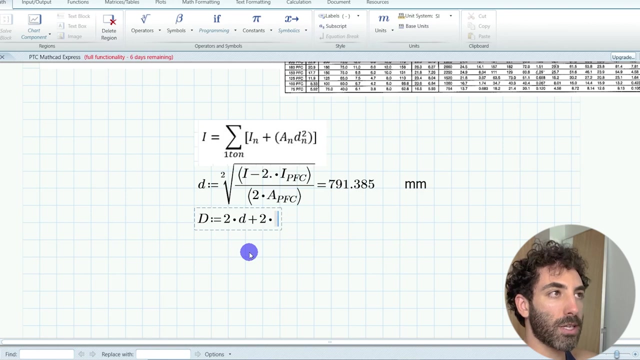 and rearranging this equation, we're going to find that d is equal to 791 millimeters. the depth of the truss is 2 times little d, plus 2 times the centroid distance, xl, which works out to be approximately 1.7 meters. right, so let's say 1700 millimeters. 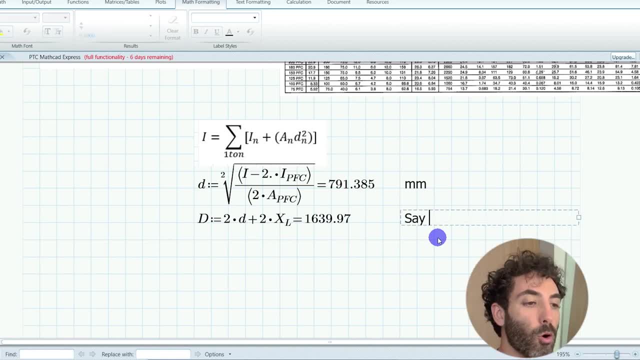 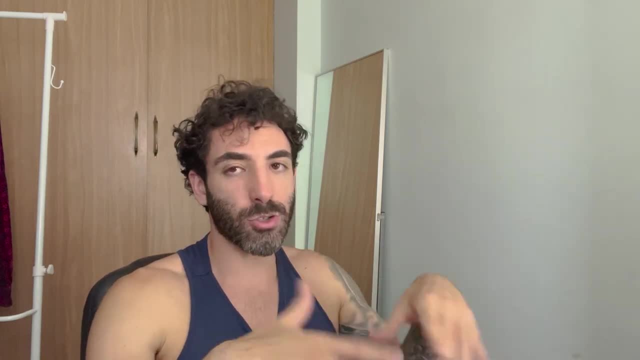 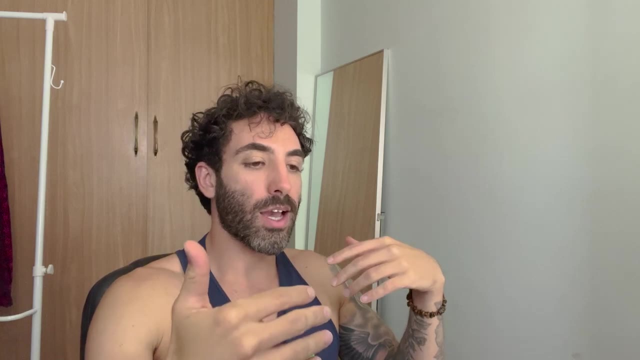 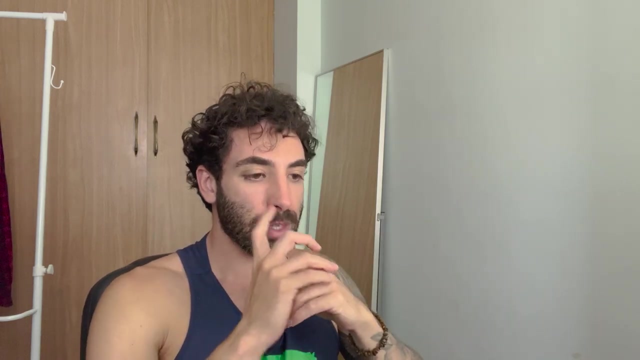 so great. now we know the depth of the truss, which is pretty much what the architect wants to know to proceed with his or her design. and this was a quick and easy concept design, and what we're trying to do here is to make you a more efficient engineer. okay, in the next video we're going to design the 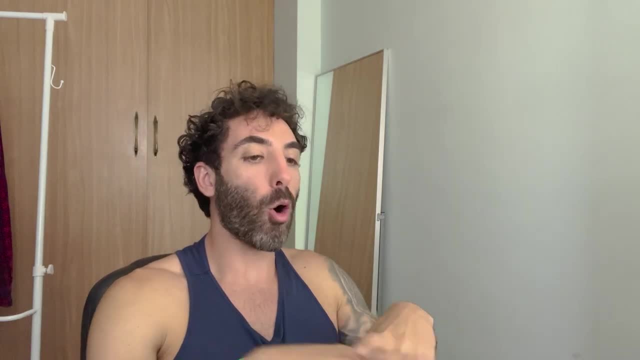 members in compression and tension, and only then we're going to open the software and verify our calculations and make sure all the numbers are correct. okay, so stay tuned.